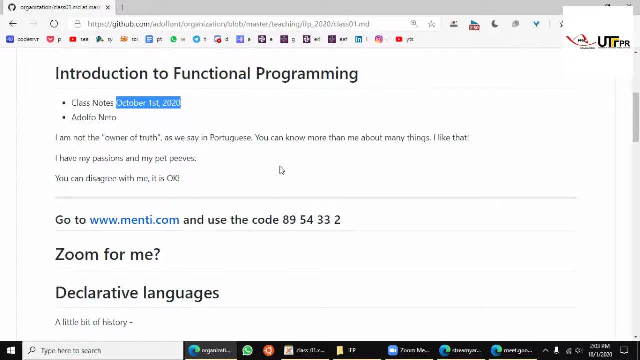 of Technology, Paraná, Brazil, here in Curitiba. So don't be afraid to say that I'm wrong, because I may be wrong And also I have my passions and pet peeves. so some things I like, For instance: 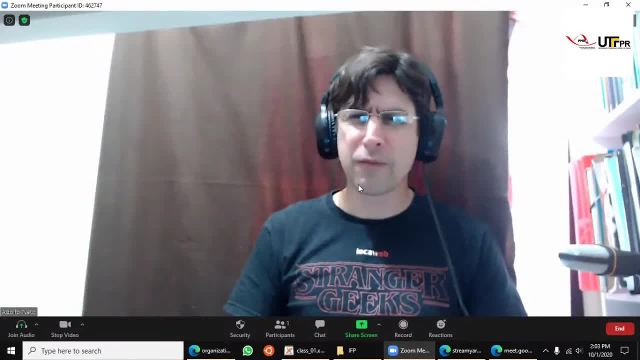 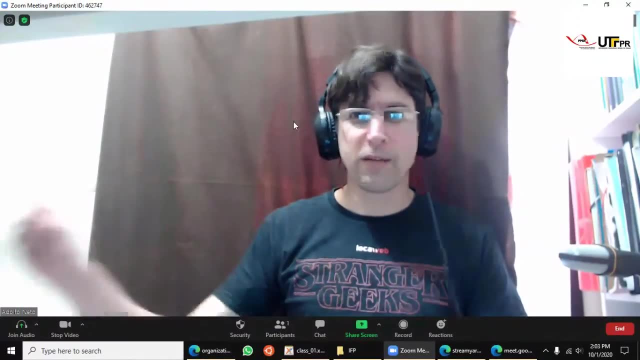 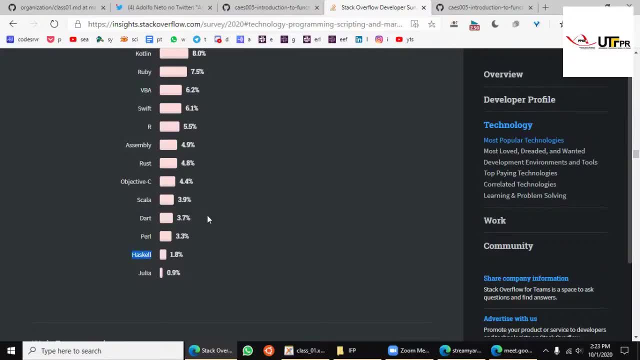 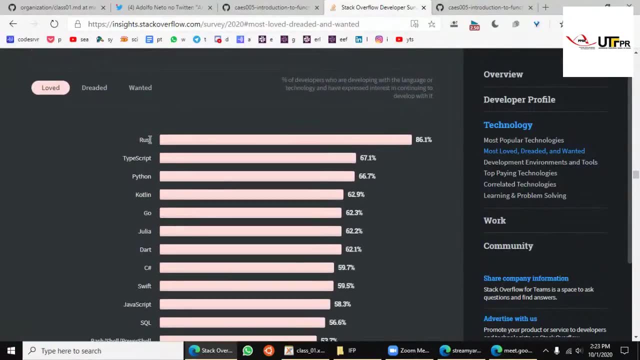 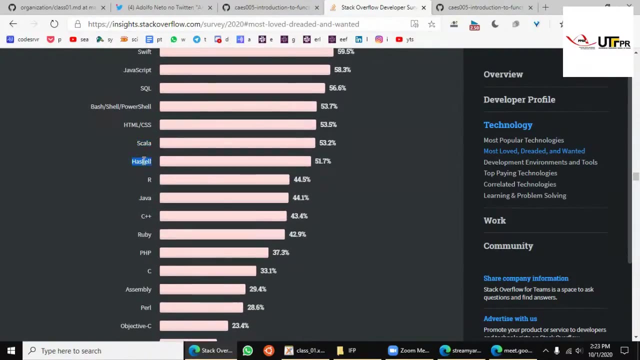 be afraid to say that. So don't be afraid to say that. So don't be afraid to say that. So don't. haskell again. uh, there is this. the most loved technologies: rust type script, python, coddling- which one here is functional, is color a little bit haskell. you see lots of people like haskell. 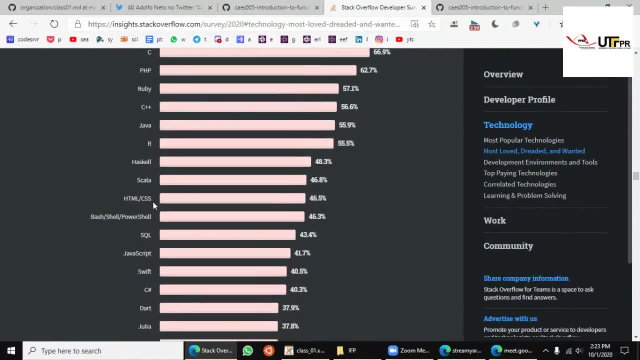 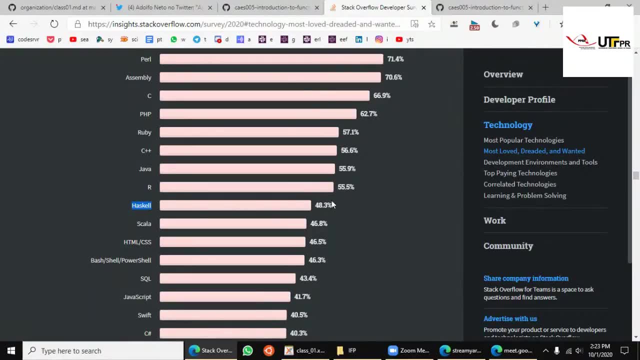 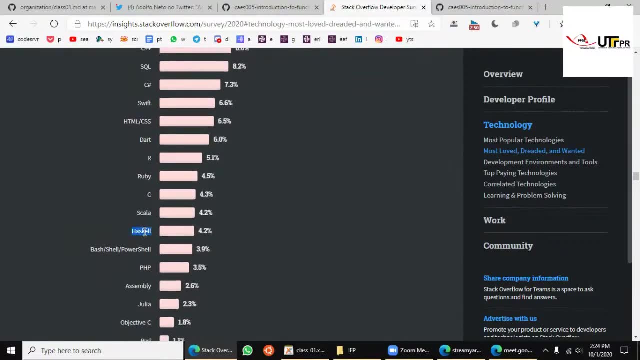 actually love. some people dread, oh see, no, not many people dread. ah, many people dread haskell and wanted it's the people that want. only 4.2 percent of people. they want to program in haskell, and i also like to see this. uh. 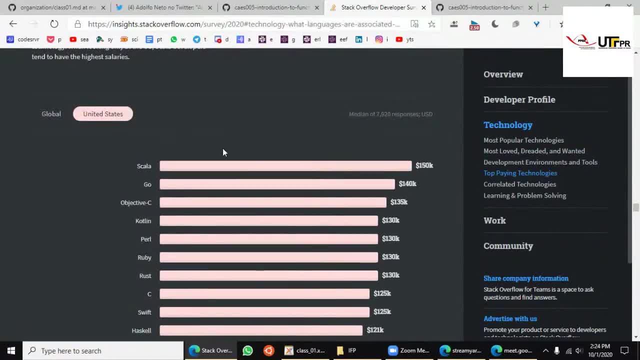 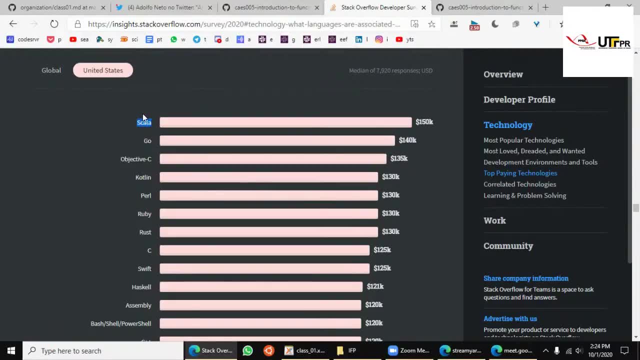 the part of on the salaries, because you see scala, which is a multi-paradigms program, functional language. if you are a scala developer in the us, you can earn as much as is you can a median- it's not the average, it's median- of 150 000 yearly. so this is a yearly. 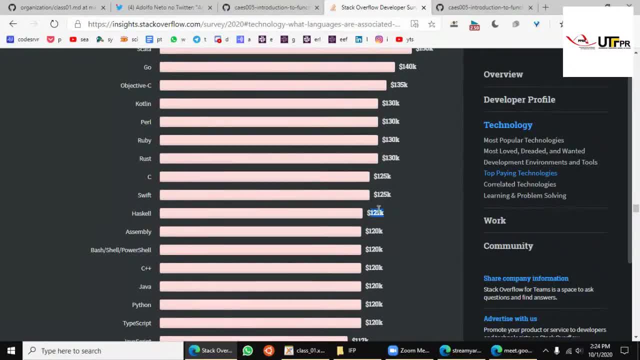 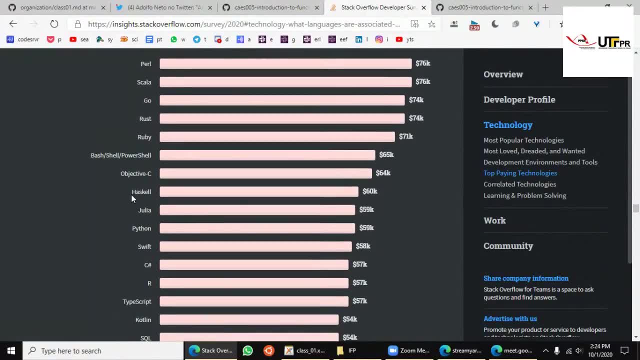 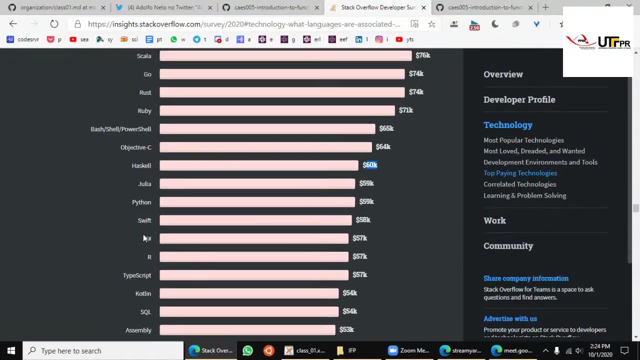 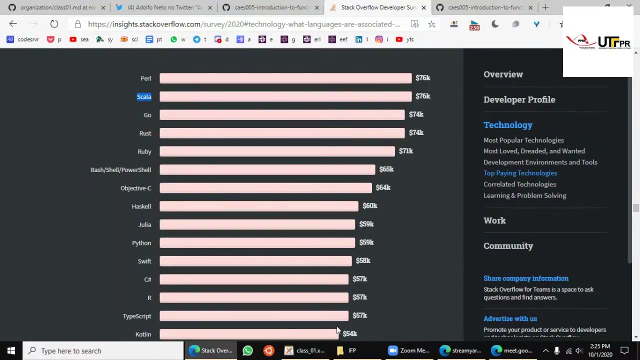 salary, which is quite good: haskell one, two, one, and these are the only functional, and here in the world it's 64, 60k for haskell, which one was the other one. so you see, it's possible if you, if you specialize in ah, this, this. 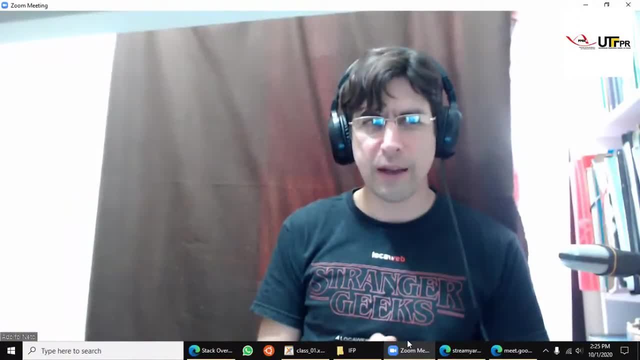 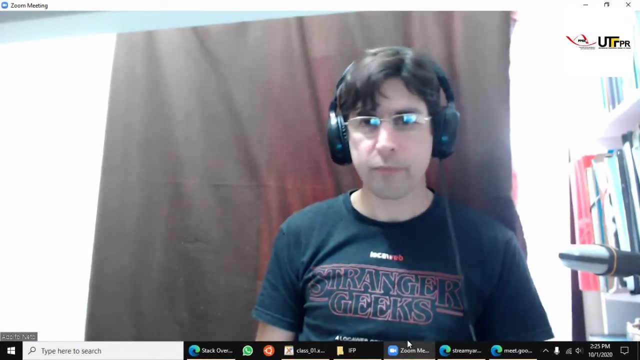 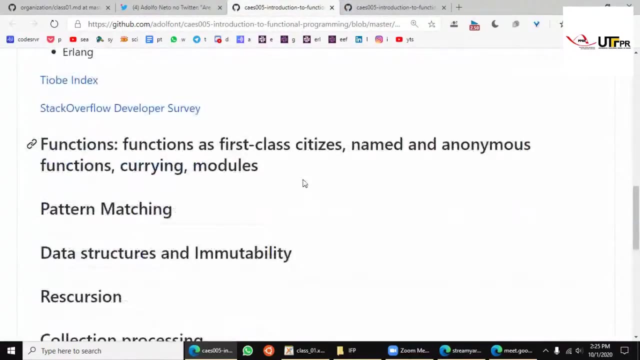 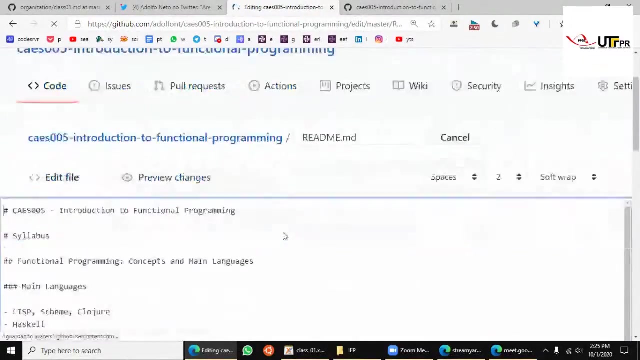 this survey was from 2020. in 2019, elixir appeared there as a with a very good salary, so it varies from year to year. and what else? ah? what are you going to see here? oh, it's, it's nice that i can change here, because 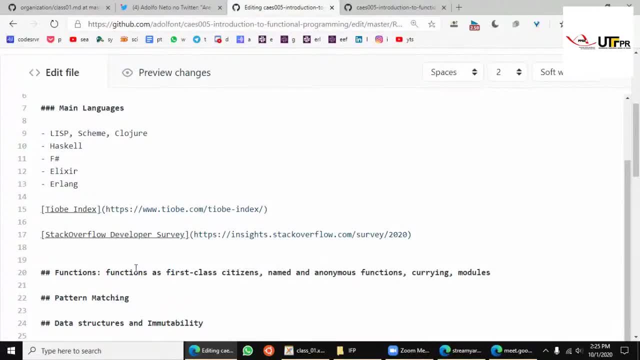 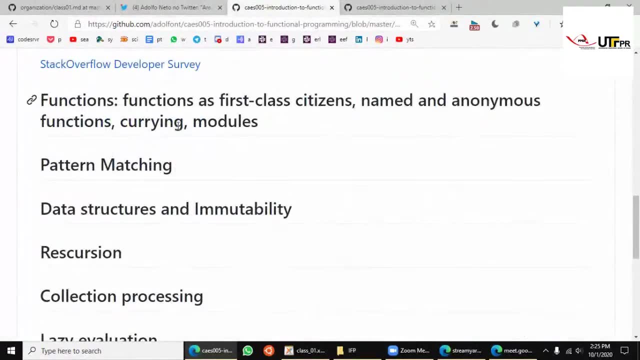 it's wrong. it's functions as first class citizens, and we are going to see functions as first class citizens and we are going to have functions as soon as you want and we are going to have students. indeedHis is another種 of issues, so you can see a lot uh, what uh to you. 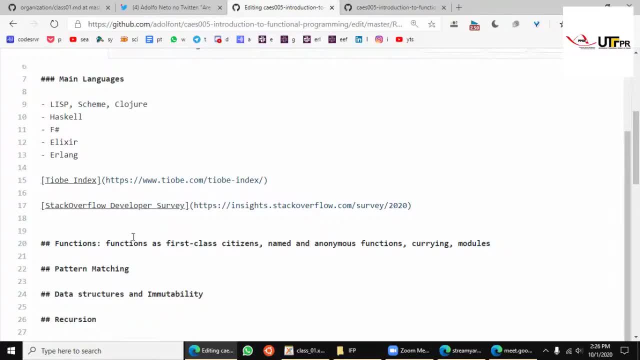 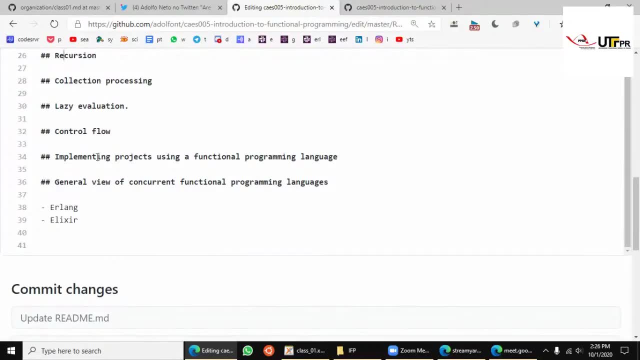 like to talk about for sure for the future of the program, variations or, like you know, uh, what's come under sub module're gray or blue or whatever. what are you going to see? um, another useful thing to to do on this call from sc: Additional Underlay. 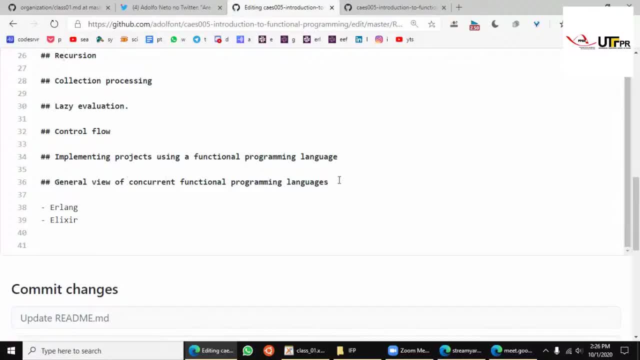 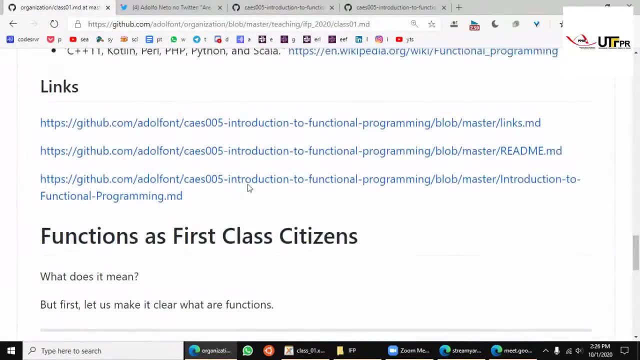 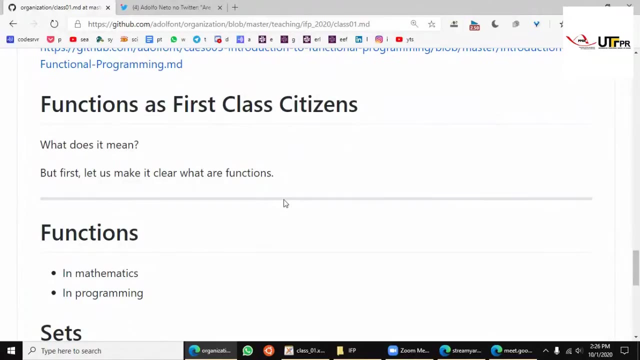 two, get your job done. Another interesting thing is this: the search engine correct is a full-time Battle account. oh okay, Ah, yes, heck, uh sorry, of concurrent functional programming language elixir in erlang, so let's go back to here. so this one i have already shown you and function functions as first class series. what does it mean? 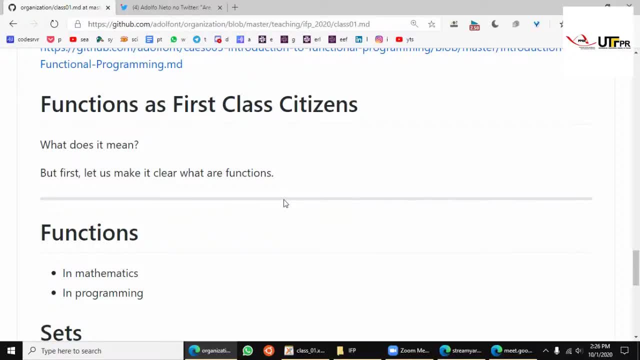 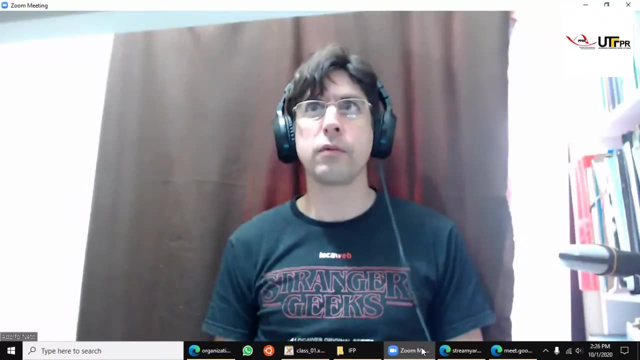 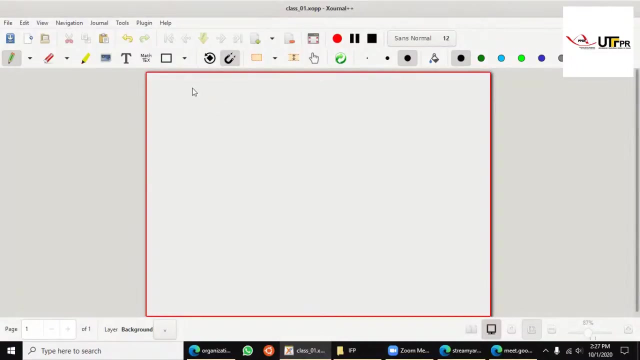 so first i have to show you what are functions in mathematics and in programming, which is different. they, these are different concepts in these two knowledge areas. so i'm going to show you a little bit how, how i see what's a function in mathematics. so in mathematics we math, and mathematics is difficult to say for me. 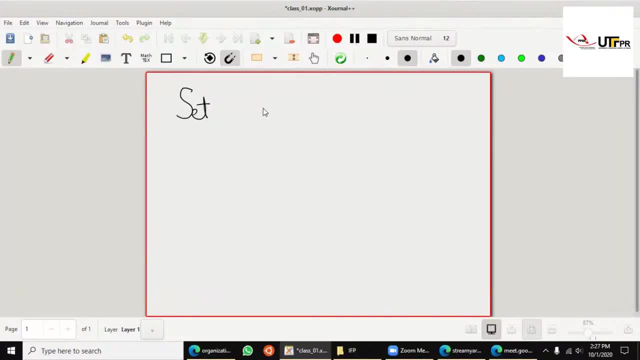 in math you have the concept of set. what is a set? a set is, for instance, let's get, if i have the set a, which contains three elements: a, b, c. a set math can have zero elements, one element, two elements, three elements, infinite elements. so i have the set a and the set b. 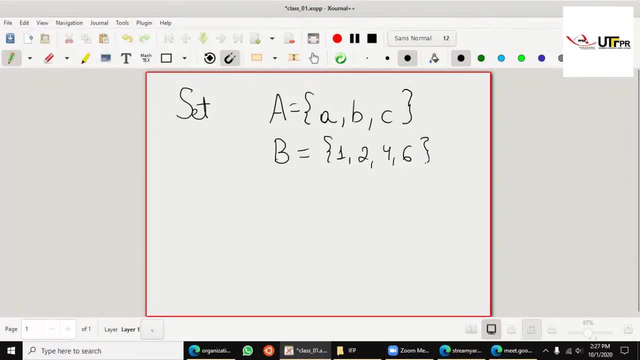 one, two, four, six. so now we have two sets, a and b. i'm going to draw them here because it will be useful, so let's let me put here A, B, C. this is the set. capital A and B is 1,, 2,, 4,, 6.. 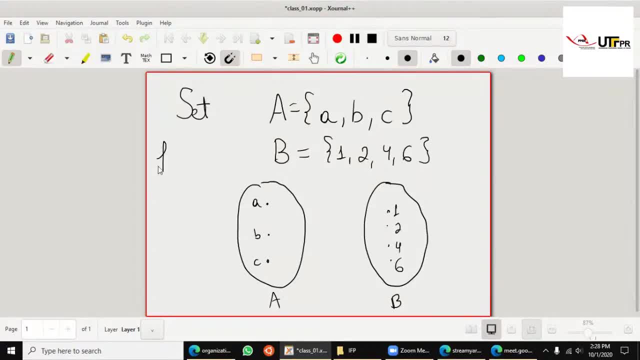 So if I say that I have a function F from A to B, what does it mean? Let me choose a different color. It means that for every element of A, I can associate it to one and exactly one element of B, For instance for this F. F of A is 1.. 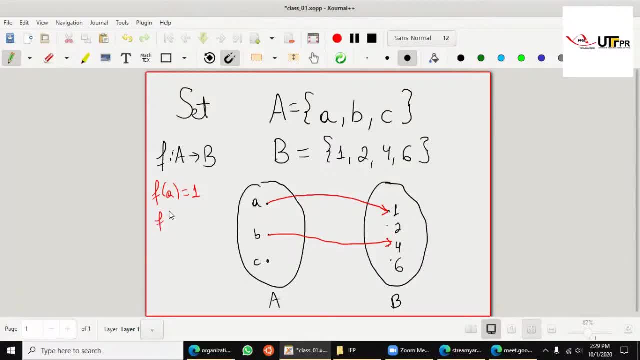 F of B is 1.. F of C is 4. And F of C is 2.. You see 6 is alone here. That's okay. I can have if it's on the right side here, it's okay. 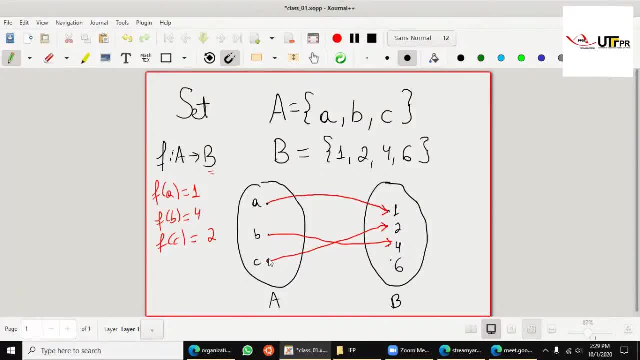 It can be associated to no one here. But if I had, if C was not associated to, to 2 or to 6 or to any one, then it wouldn't be a function. In order to be a function, I have to associate every element of the domain set. 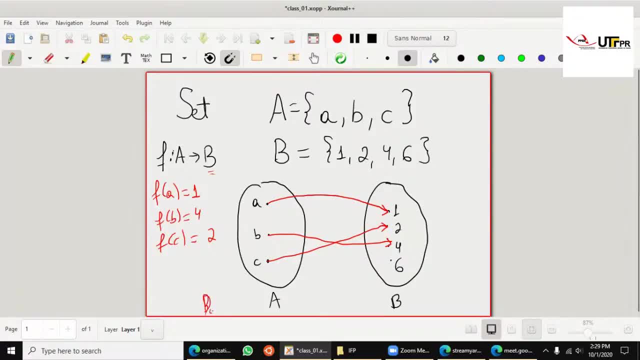 We say that this is the domain. Oh sorry, Domain and image. Every element of the domain is associated to the image, But not every element of the image is associated to an element of A. It's the destination of this association. So this is the basic idea of functions. 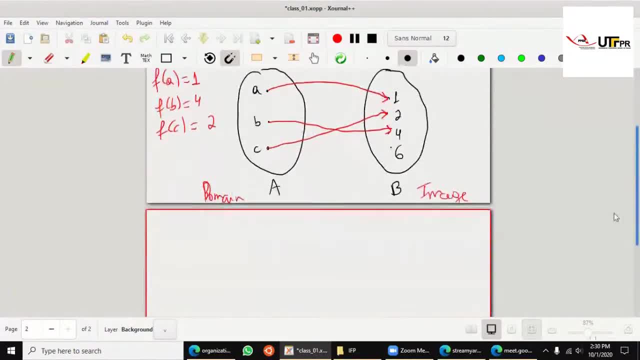 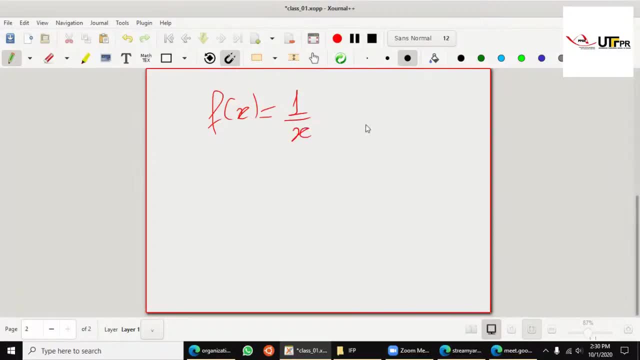 But this is interesting because, for instance, there is this function in mathematics, that's- And Let let's say that this function is from the, the set of natural numbers, to the set of natural numbers, F of 0, which is the F of 0? 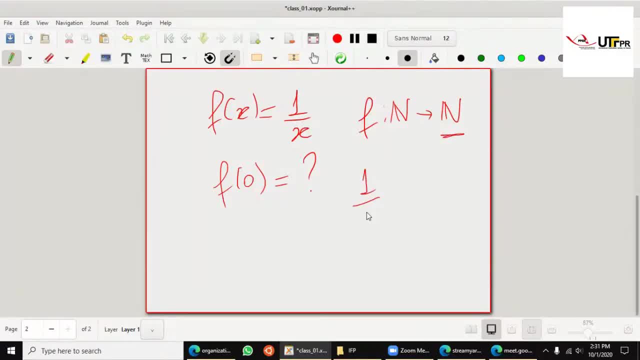 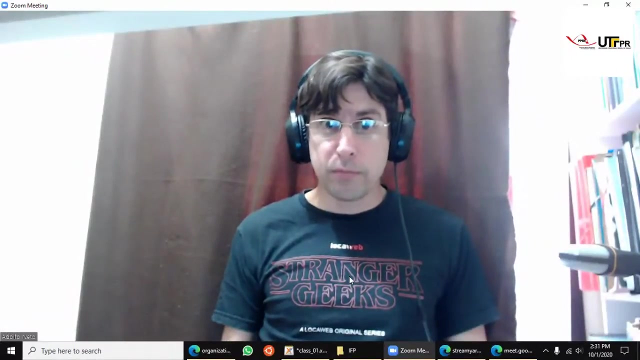 There is no natural number which is equal to 1 over 0. So this is not a function, Right? Not a mathematical function. So that's the the the the question. here We have a mathematical definition of function that, even for some, some things that are quite usual for us in our day to day- 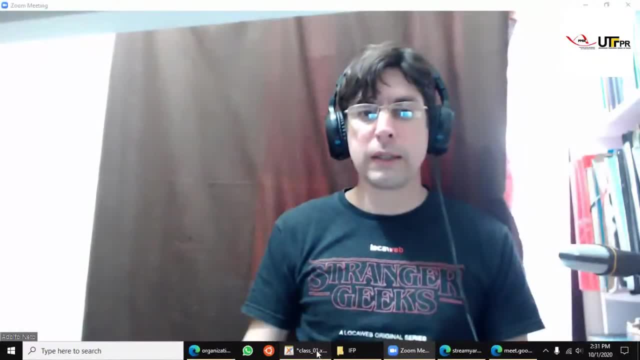 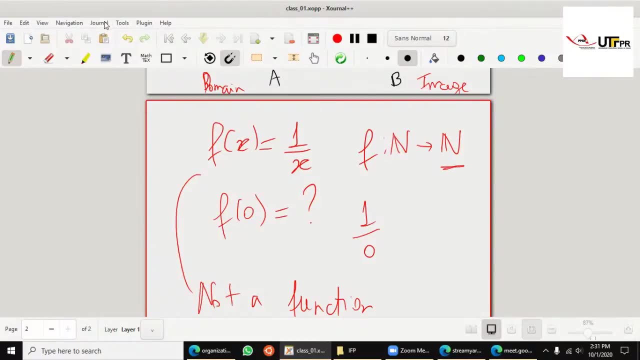 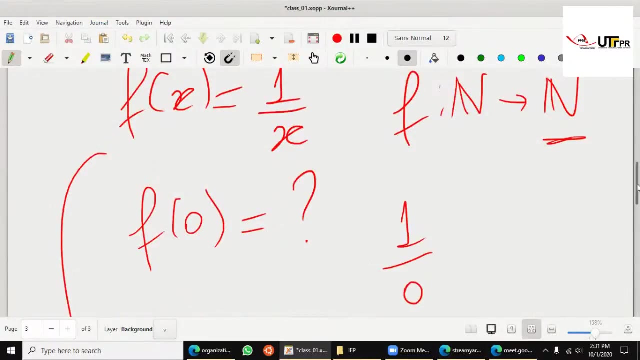 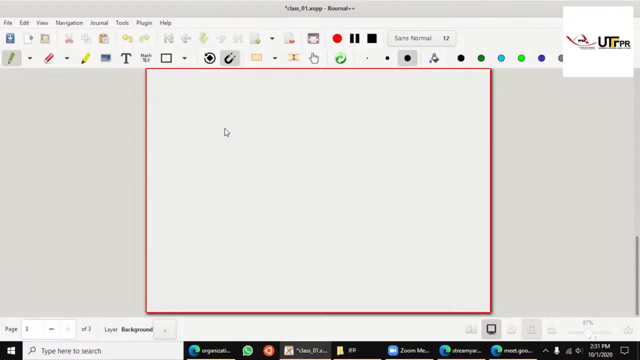 You don't, you don't use it. So in computer science It works, It works, It works. It happens too. So I'm sorry I have to include here a new page after Yeah. So in computer science we have a rather 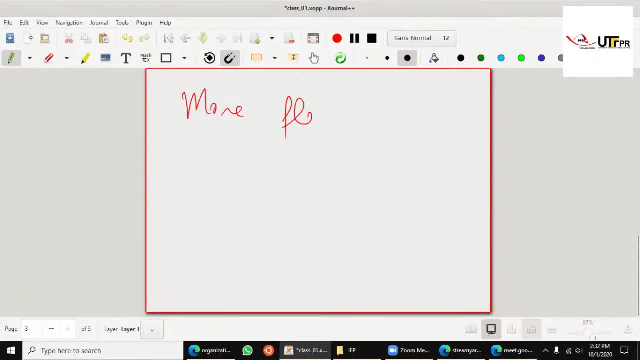 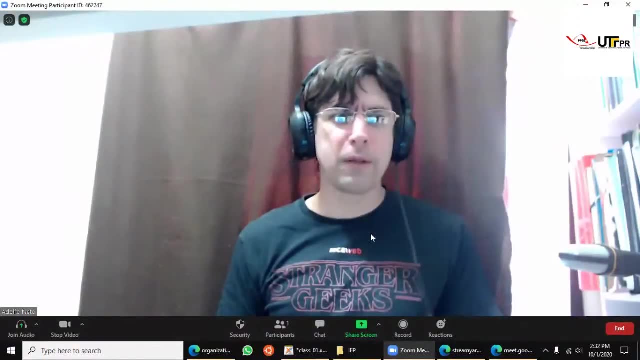 It's a more flexible, more flexible definition of what a function means. It's a more flexible, more flexible definition of what a function means. It's a more flexible definition of what a function means. I don't have the time to explain to you concepts such as computable, non-computable functions. 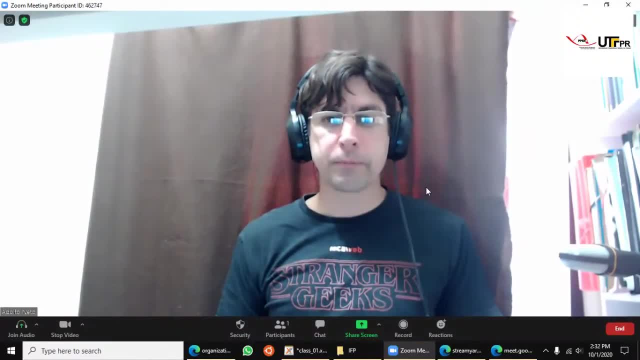 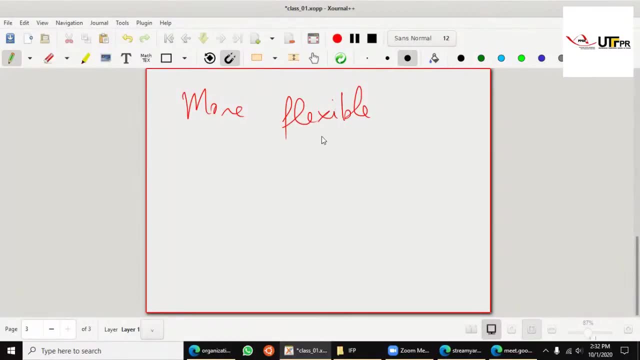 It's not part of this course And but you can have some In some programming languages a function. you can have something like this in some programming languages In some programming languages, a function. you can have something like this in some programming languages. 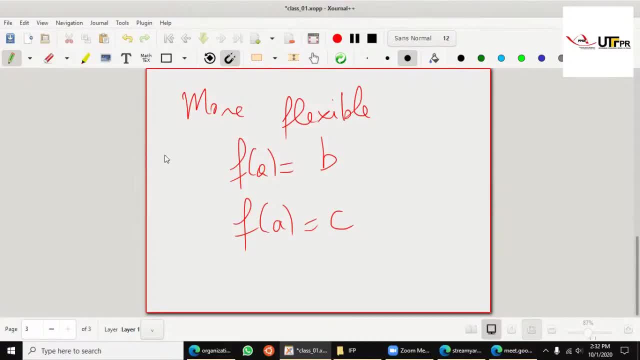 See, Now it's 2.32 pm, And let's see. And let's see, Let's see If I, if I ask the computer to calculate the result of this function, f with e, oh sorry, with a, on 2.32 pm, the result is b. 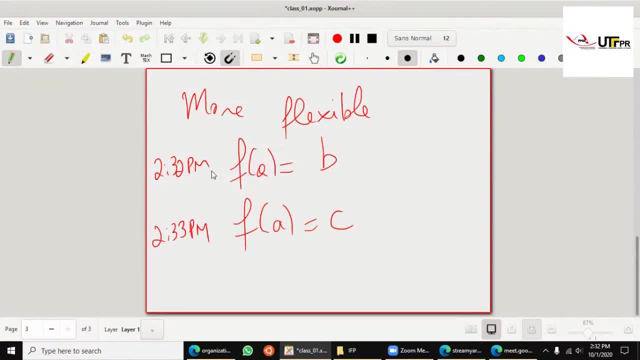 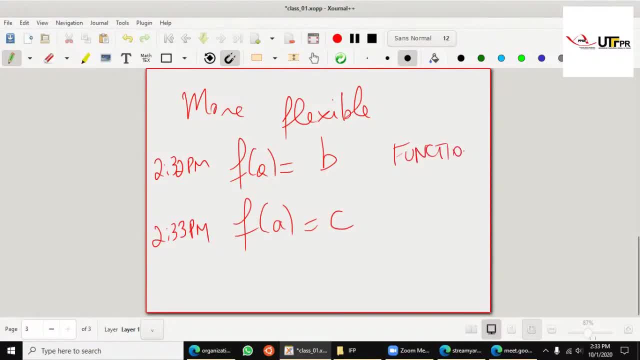 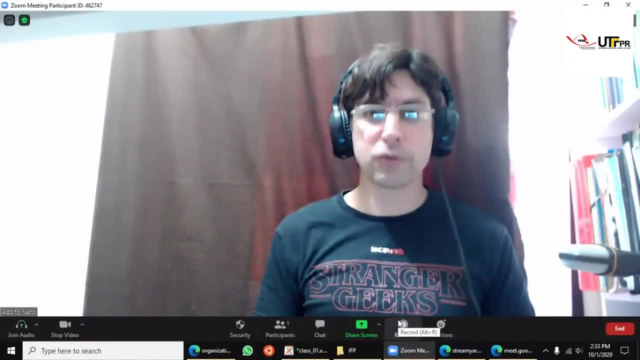 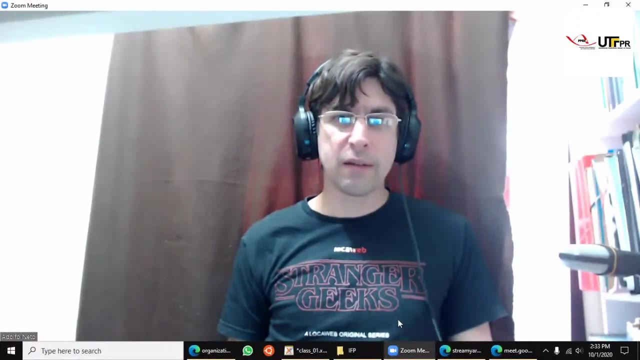 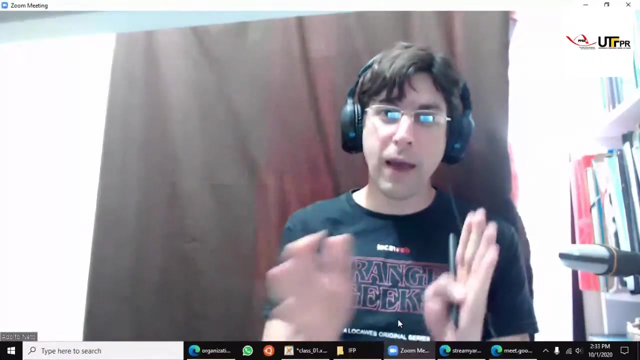 This is a function for programming people, It's okay. Some people say this is a function, So it's not a big problem. But the main question here is that when you are talking about proper, about functional programming languages, our functions are more like math functions. 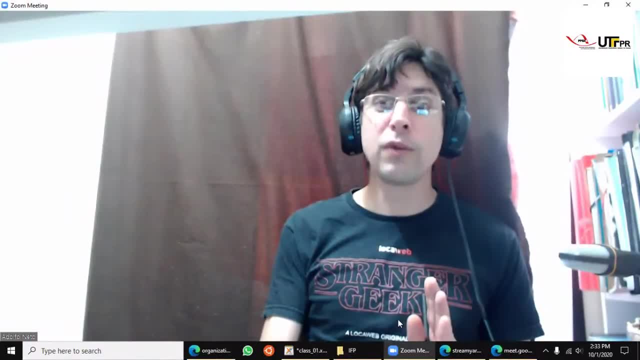 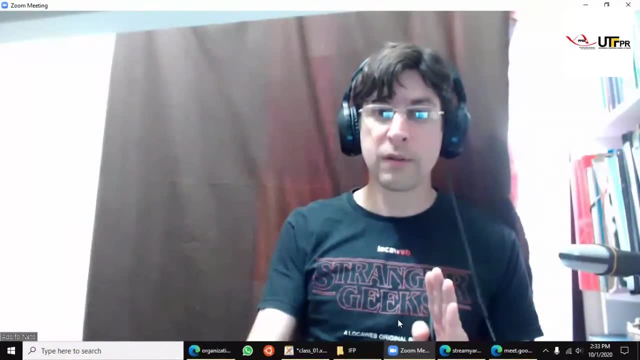 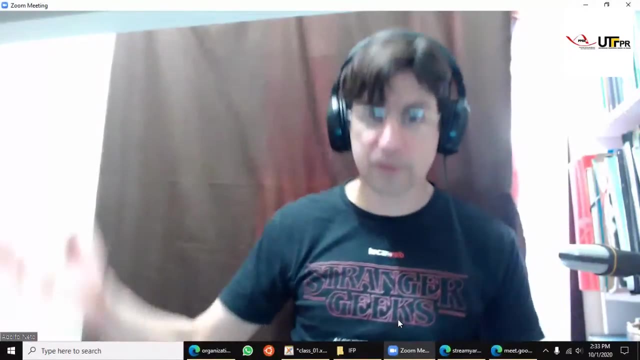 When we give the same input, it returns the same output. So that's the basic concept here: The same input, the same output ever Doesn't change in a different time in a different configuration. So I believe this is going to be become more clear. 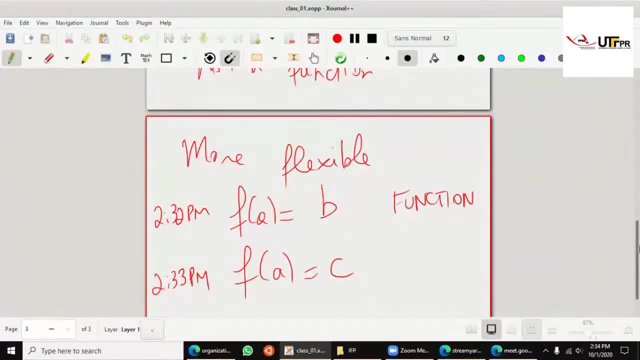 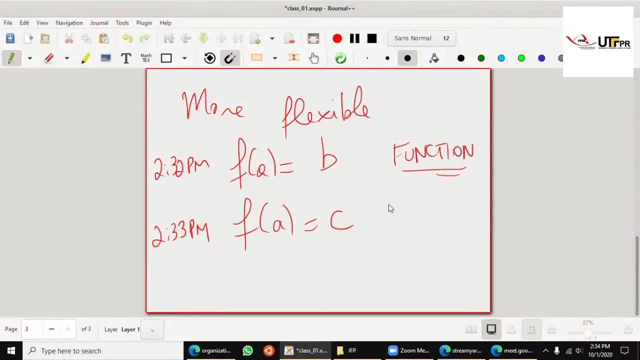 when you present. but do you remember that thing about purely functional? So the question is that some language, even Elixir, some functions, even Erlang, some functions that we call ah, this is a function then, but they don't respect this. 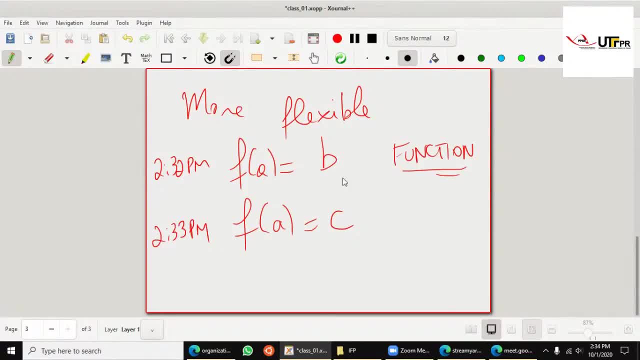 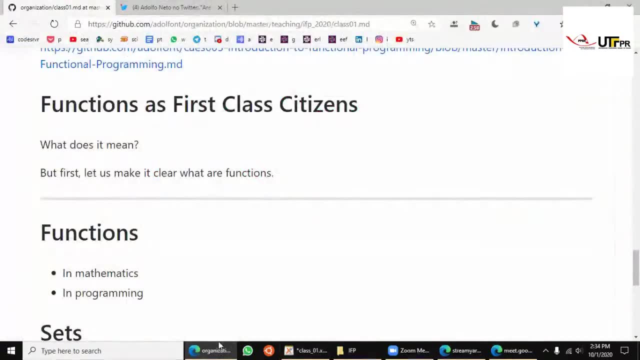 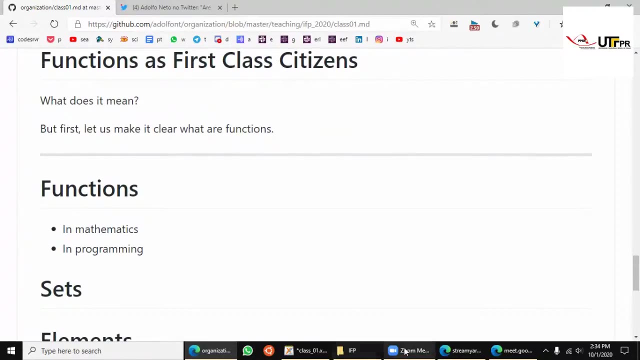 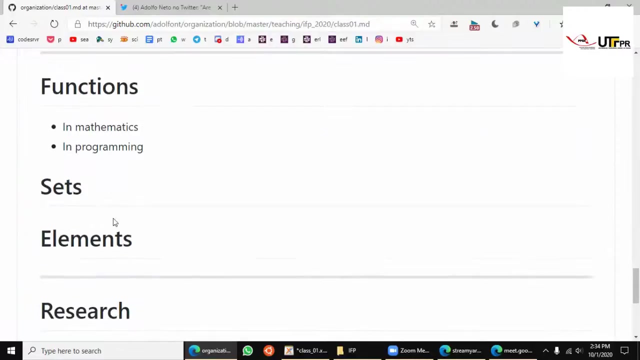 They have for us the same function and the. they give different results at different times. So this is the, the, the first thing, So our functions. in functional programming language, the functions are more like mathematical functions, And so I have presented these here. and the first idea. 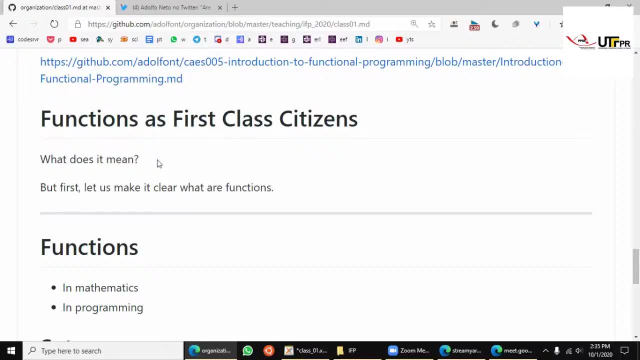 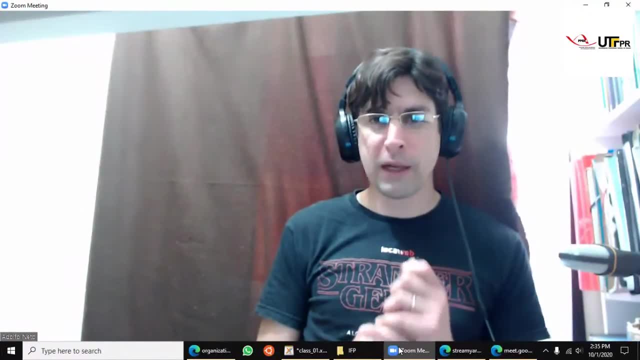 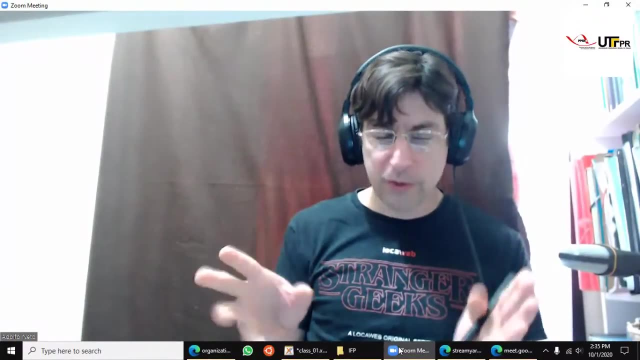 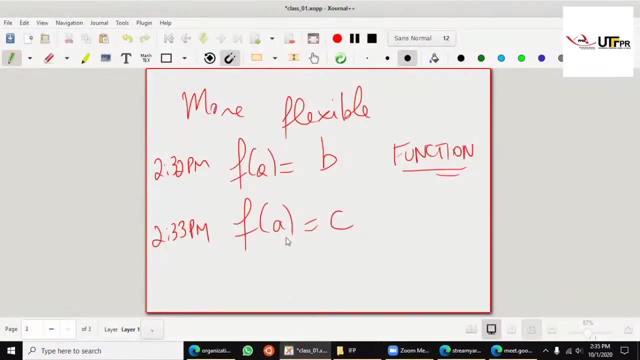 that I think it's also important, for I see that most of you have some background in programming. usually, in most programming languages, you can define a function, but you cannot. you can define a function. the function can receive many arguments, for instance in our example here: 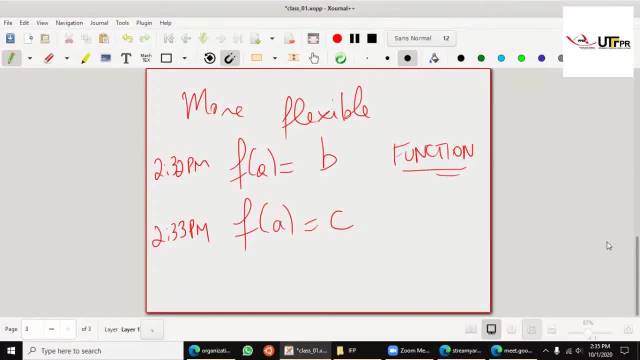 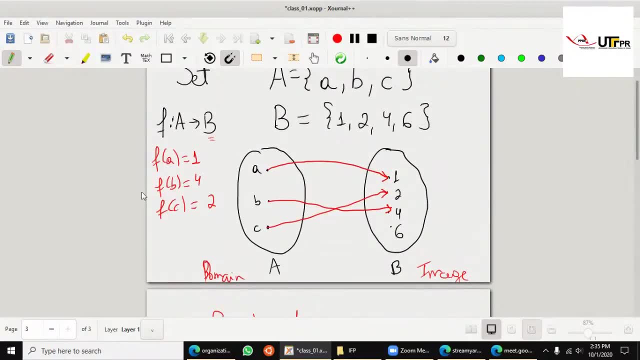 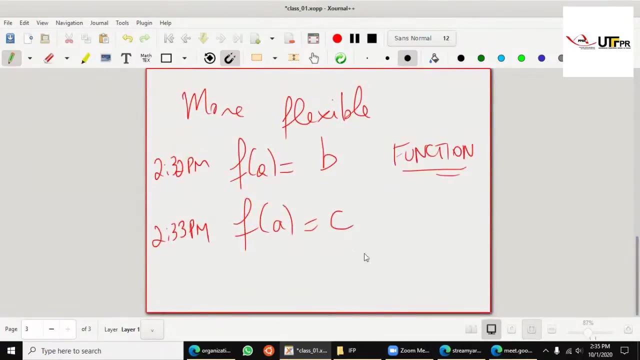 A is an argument, A is an argument here and, sorry, here A, B and C are arguments. 1, 4, 2 is the result and most, most programming languages you can have. I can say f of x is x plus 2, but I cannot say: 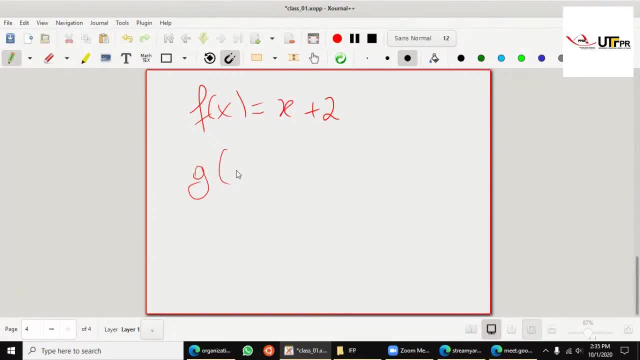 oh, there is a function g that receives y and do something. for instance, this is a function that receives x and returns x plus 2, and this is a function that receives y and applies that y to 3. so in this case, g of f would get f. 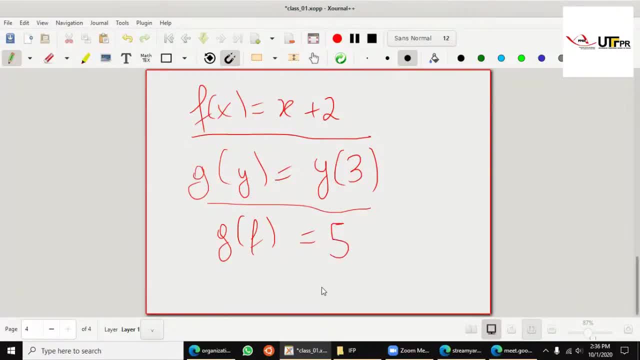 and apply to 3. 3 plus 2 plus 2 is 5. so you see this, I have passed a function as a parameter parameter. so most programming languages do not allow this. so this is the idea of this is the basic idea of a function. 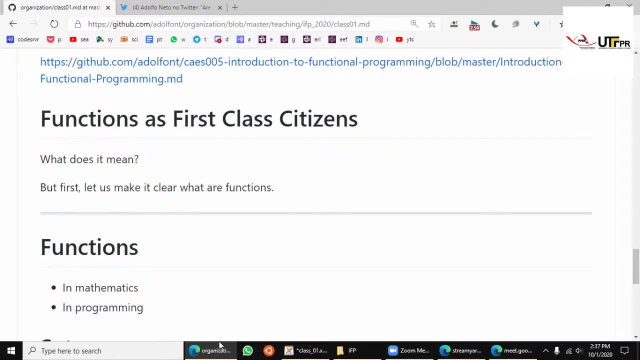 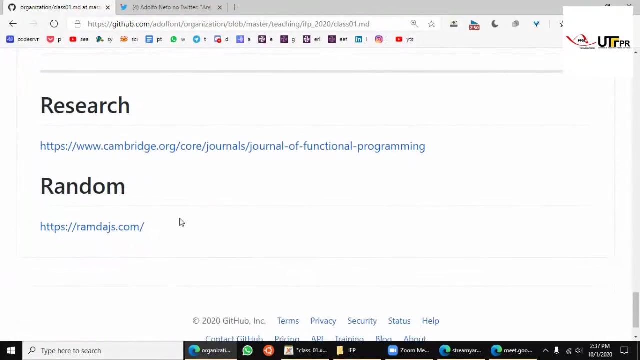 as a first class citizen. in most functional programming languages- I believe in all functional programming languages- you can define a function, you can pass it as a parameter, you can return a function from when you apply a function. so that's the basic idea, something that I, so I'm going to explore these concepts a little bit more. 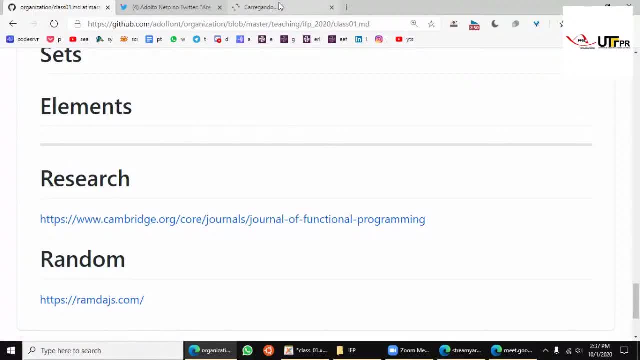 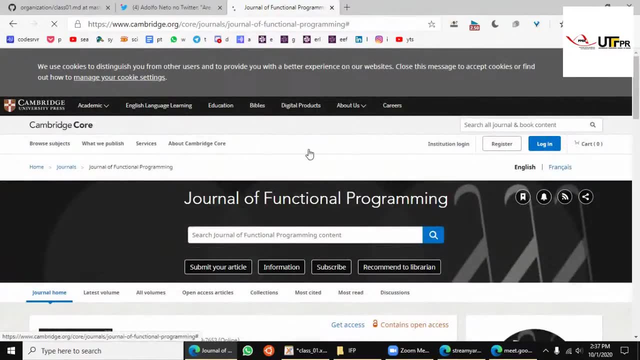 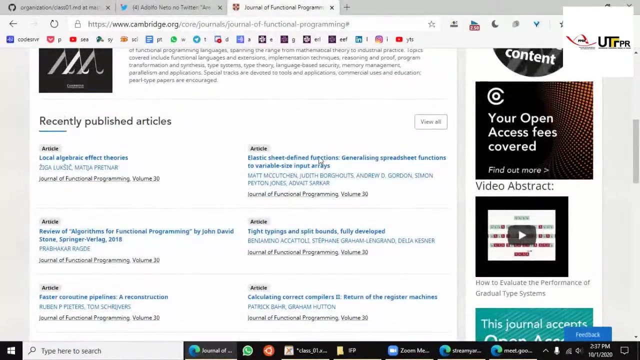 a little bit more. uh, something I wanted to show to you is that there is a lot of research. um, this is. this course is part of our master's course. so there is this journal of functional programming. so there is very advanced content on functional programming. we are not going to. 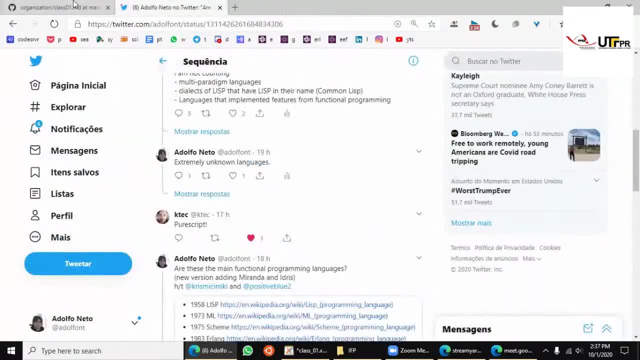 to go there because this is an introduction course. this is an introduction course, so this is an introduction course, so this contents the course, the course. so there is非常 advanced content on functional programminglightning. we are not going to go there because this is a lexicon houses. so, apart from programming means data, where data 지�μın lá ב remnants of a lot of Chaos起こ, sampling tests. we are not going to go there because there is an introduction course, bi dér. 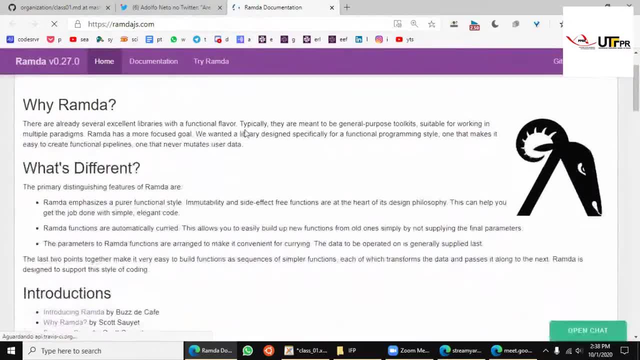 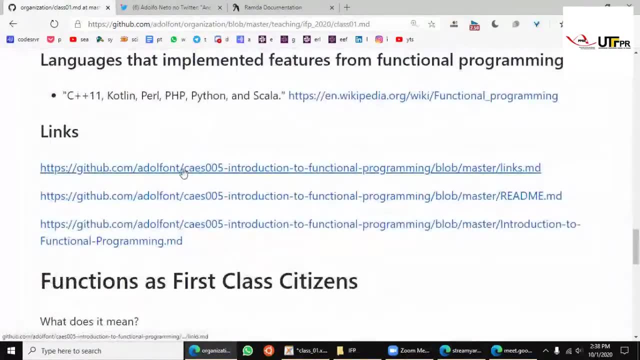 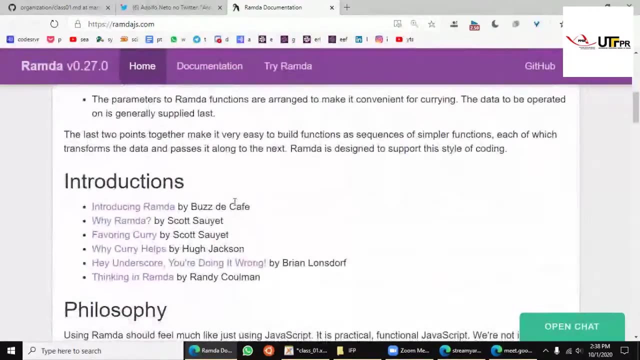 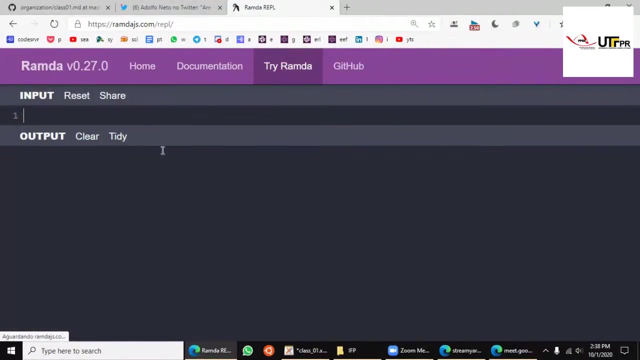 This is a point. Ah, this is interesting as an example, because this is a functional library. I had told you about the idea that language is implemented features from functional programming. This is an example I believe these guys they have. you can use functional programming with JavaScript. 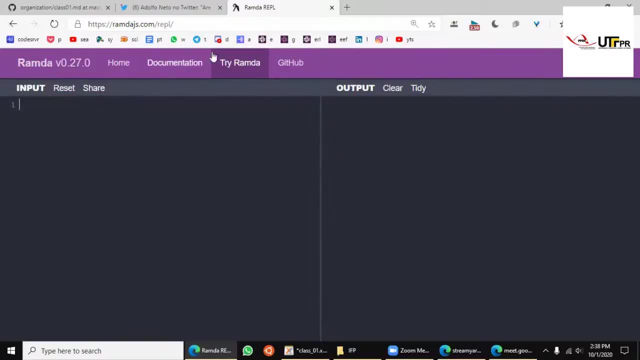 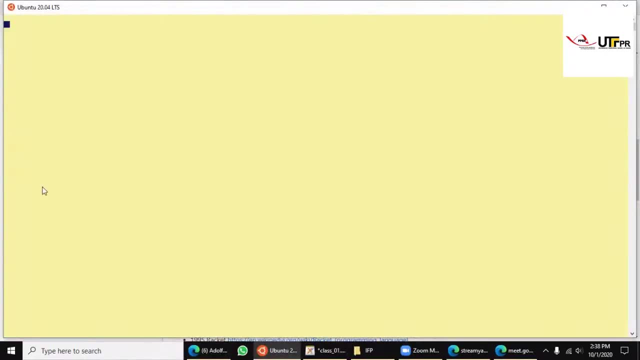 And there is no example here, but okay, let's go back. So what I want to show you now as part of this class is that the language, the functional programming language, which is not pure, that I like to use is Elixir. 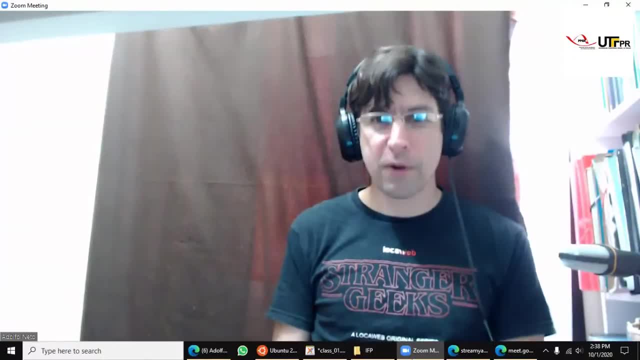 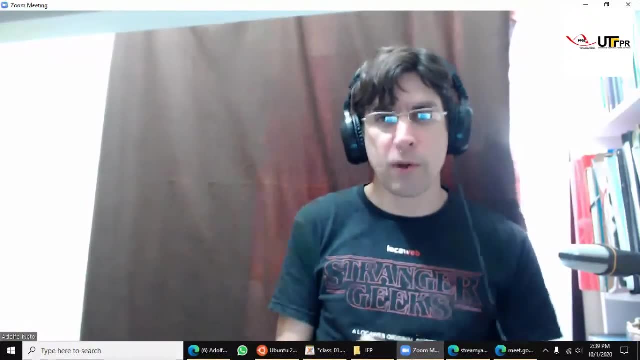 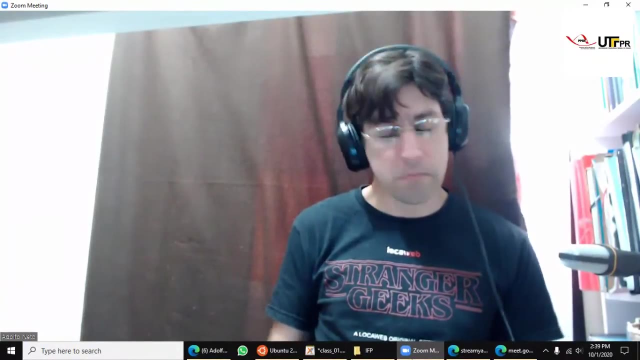 Why Elixir? Well, because it was created by a Brazilian, José Valim. I like its syntax and basically that's it. It's good for concurrent programming, which is something that can be very useful nowadays. I don't have many explanations for this. 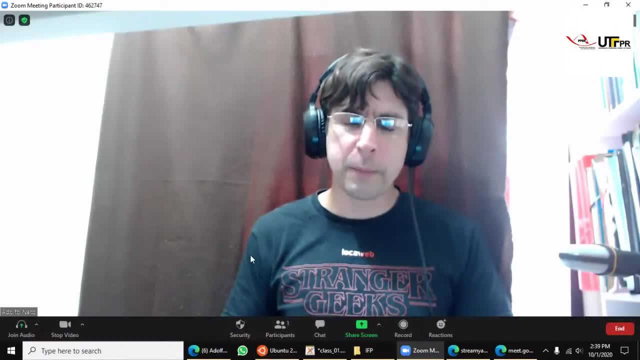 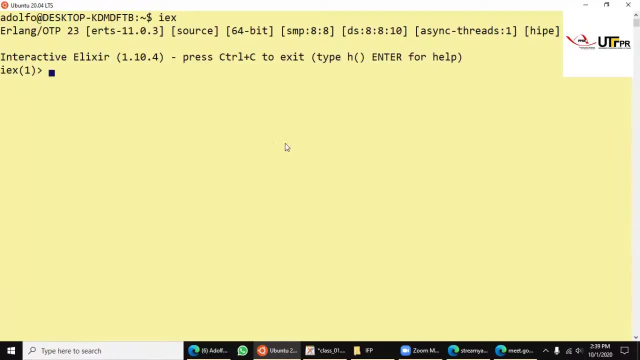 I believe most people that teach functional programming they choose Haskell, but I like Elixir, So that's why I'm going to use Elixir. So I'm going to give a brief introduction to Elixir. So, first thing, I have already installed Elixir here. 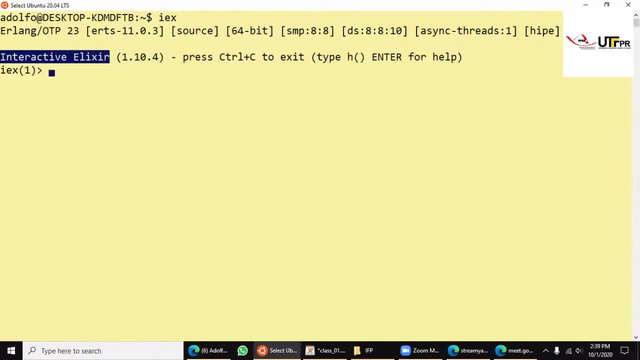 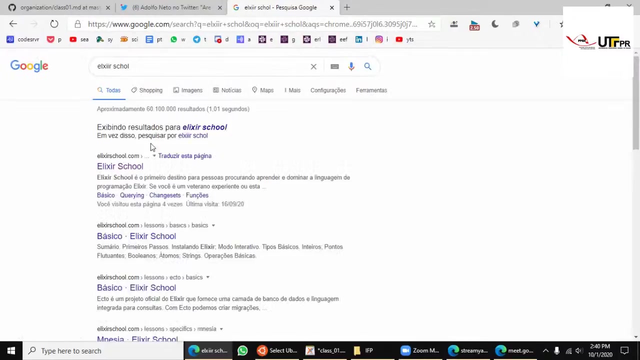 and I called the IX, which is interactive Elixir. I'm using version 1.10.4, and I'm going to show you the basic types. Ah, let me show one resource which I think is very useful. It's called Elixir School. 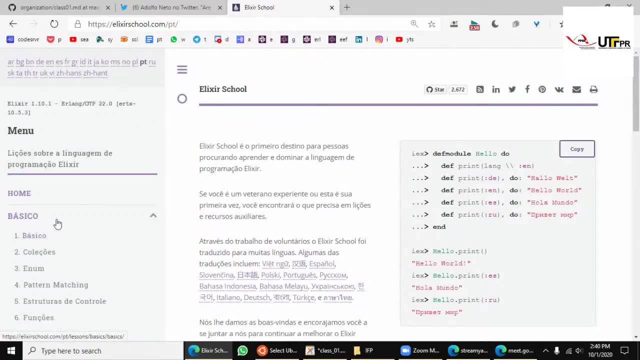 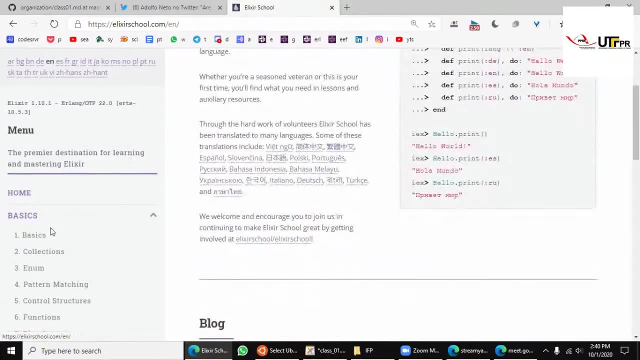 And Elixir School, you can. ah, you see, this one is in Portuguese, It's available in several languages And, for instance, when they show here the basics, they say, ah, these are the. I don't want to show you all the basics. 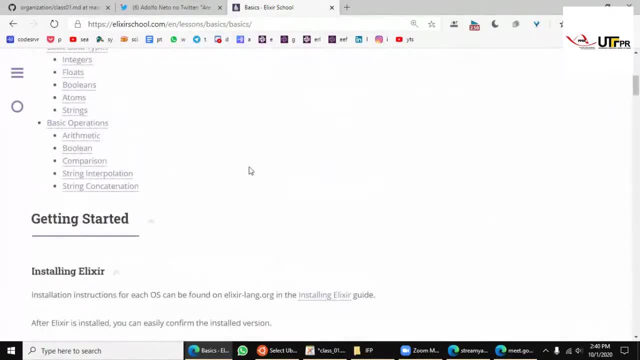 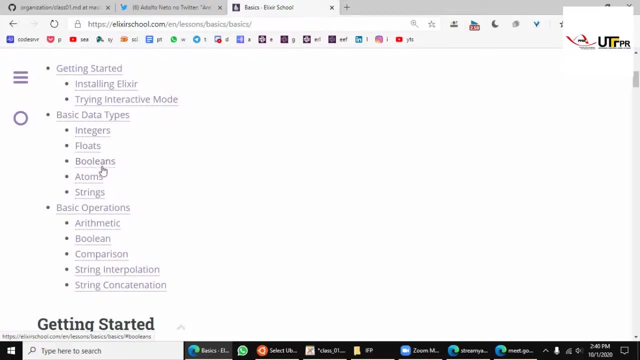 I'm going to show you how to implement it, Oh, sorry, to install it. The basic data types: Integer, integers, floats, billions, atoms, strings. So later you, you study here, but it's the basic. this is an integer number. 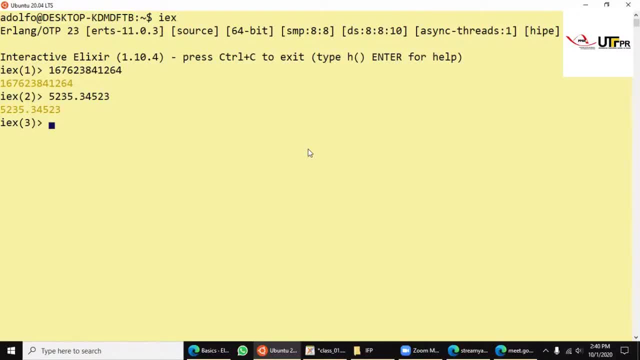 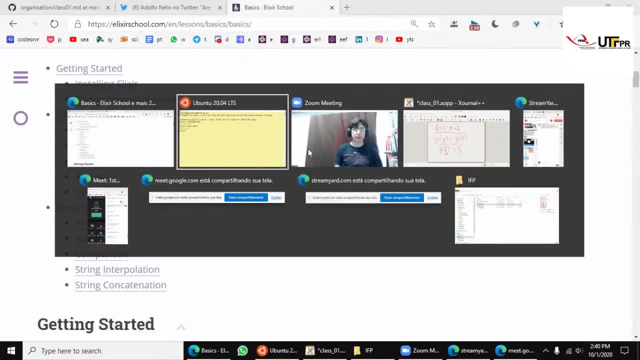 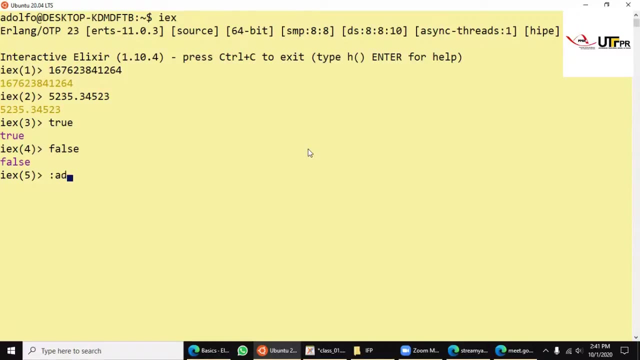 This is a float, floating point number. What's the other one? Ah, booleans. booleans are like this, true and false. Atoms are, for instance, age, name and strings. My name, Adolf. So these are the three basic types. 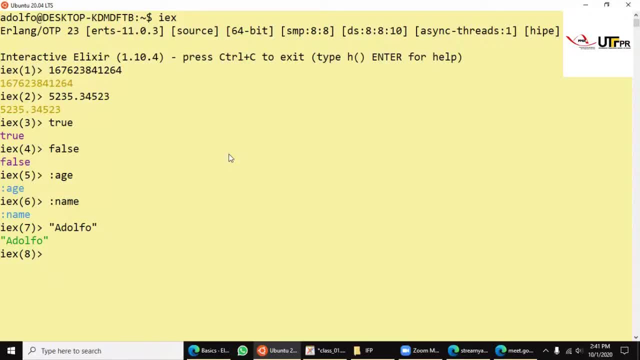 Why do I want to show this? Because this is only the start right. So let me clear here: When you open the interactive Elixir, you have already a lot of functions available for you. For instance, let me include here a string called Adolfo.